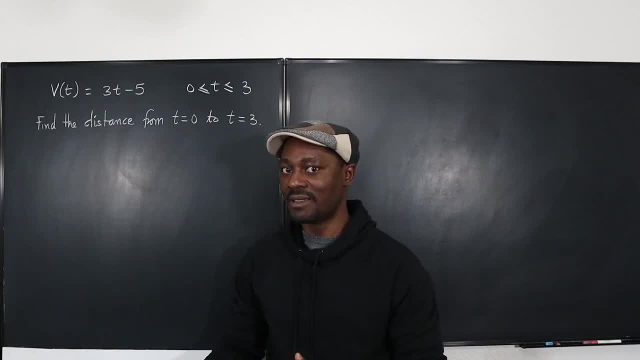 5,, which gives you 9, but 9 is not the answer. Okay, and some people have said: come on, it's a velocity function and you're going from 0 to 3, just integrate, just do this. 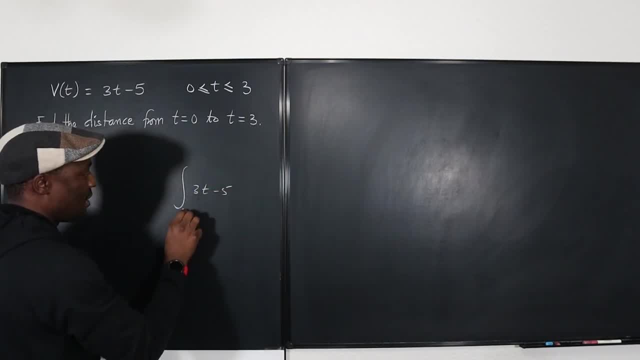 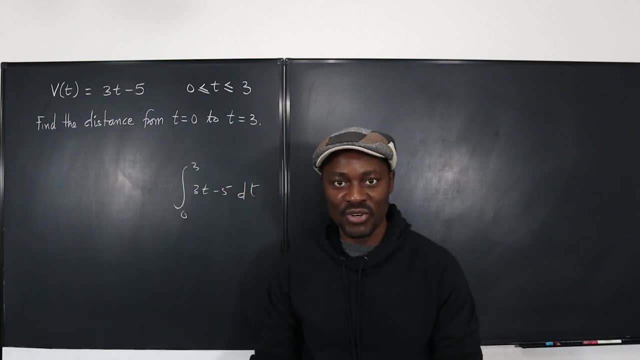 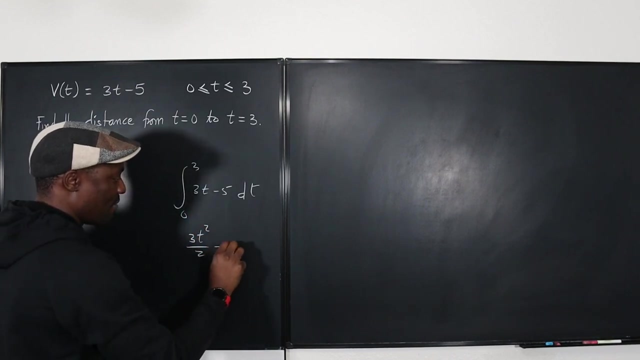 is the integral of the velocity function 3t minus 5, from 0 to 3 dt. Whatever you get will be the distance that the particle has travelled. but if you do this integral, what you're going to get is 3t squared over 2 minus. 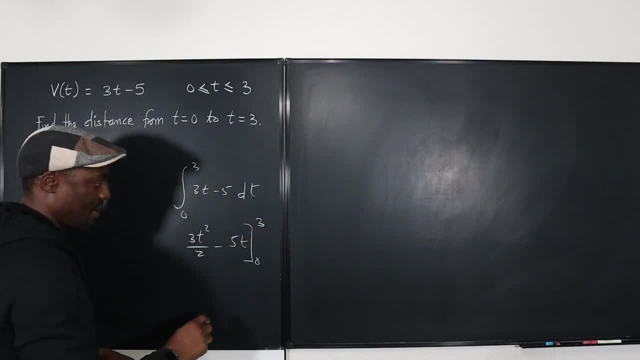 5t, evaluated from 0 to 3, and if you do that, you're going to get 27 over 2 minus 10.. 27 over 2.. Minus 10 is going to be 27,. sorry, minus 15.. Oh, it's even 15.. So it's going to be. 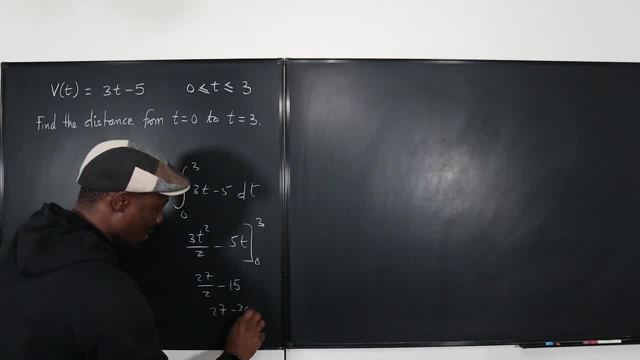 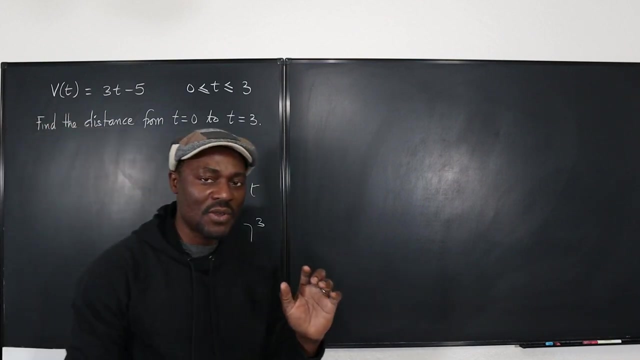 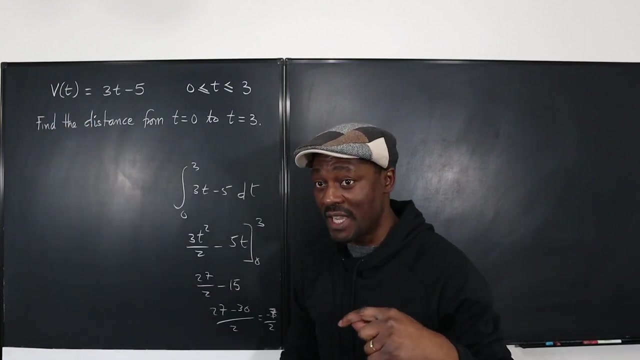 27 minus 30 over 2, that's negative 2.. Okay, this also is not correct. So what really is going on? How are you supposed to find the distance if all you have is the velocity function: Distance, not displacement? Well, if you're watching this video and these two options, 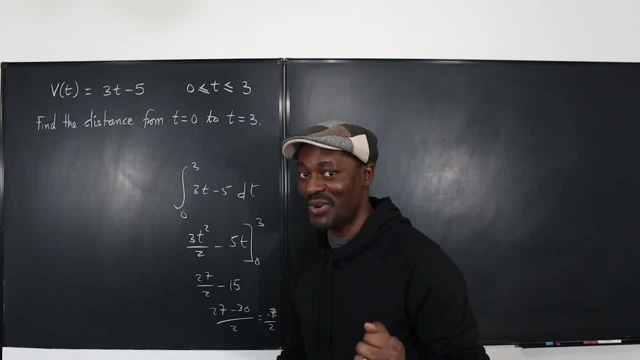 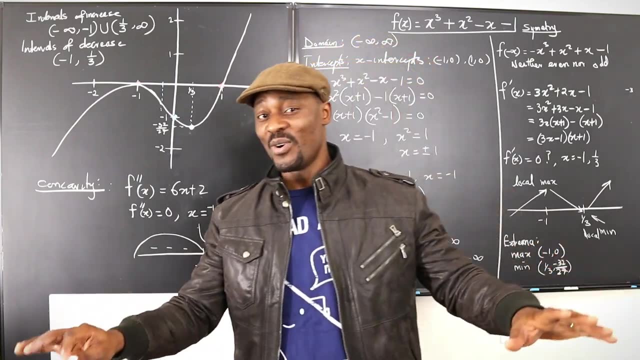 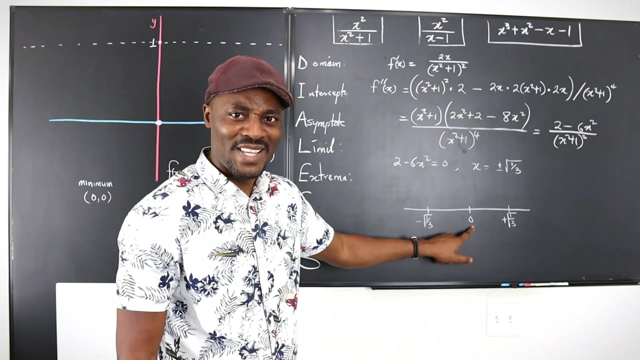 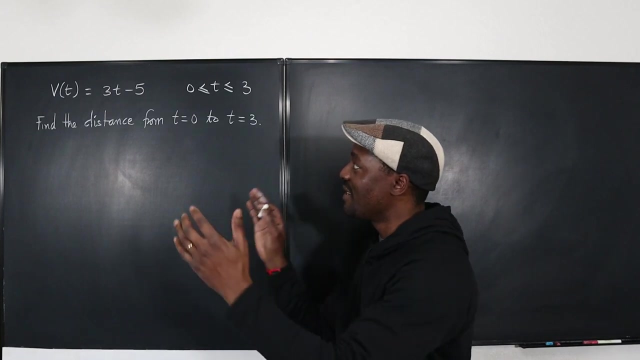 frustrate you because I said they're incorrect, then you're in for a good time. Let's get into the video. So let's go straight to the point. Whenever you get a velocity function and you're using a blender and trying to find the distance or time interval to find the velocity, remember, 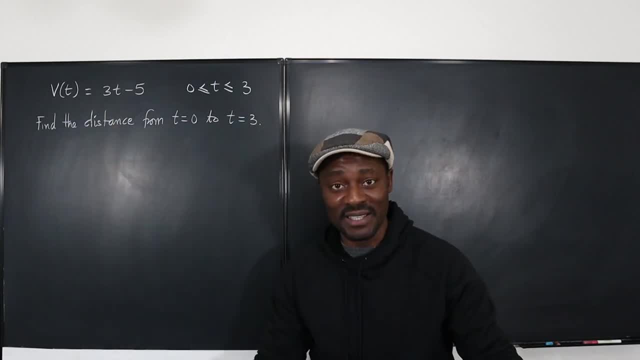 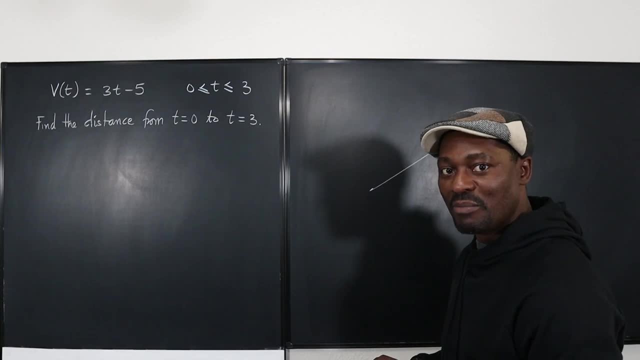 the question is about distance, not displacement, because there's a difference between distance and displacement. If you start from here and you end here, the displacement is just this. But how did you go from here to here? What if you went this way and eventually got here? 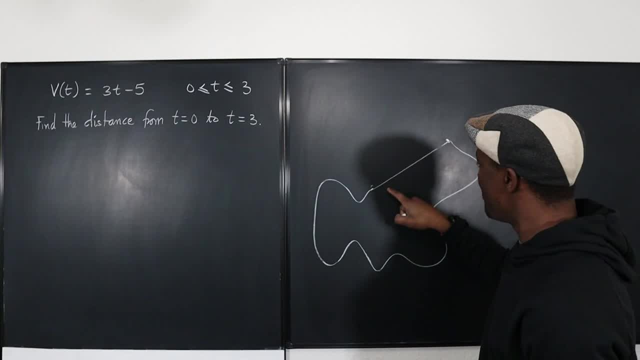 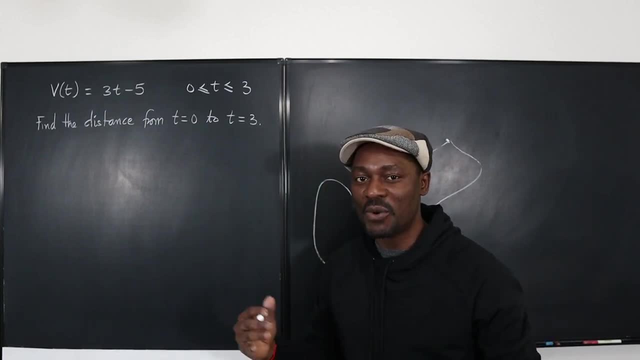 This is the distance you have travelled to get here, but this is your displacement. Okay, so a direct integration of different voltages. You can have two levels of velocity, but what of this, without considering whether you were going left or right, is going to be just this distance. 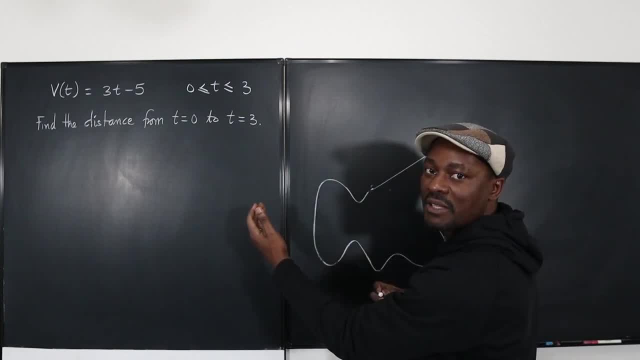 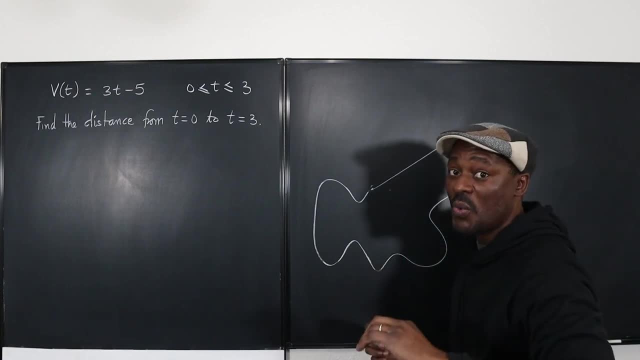 so if you went left, you're going to get a negative displacement- okay, but your distance is just an absolute value function that tells you everywhere you go, whether left or right. we're going to add up everything and we're going to get a number which is going to be positive, because you actually 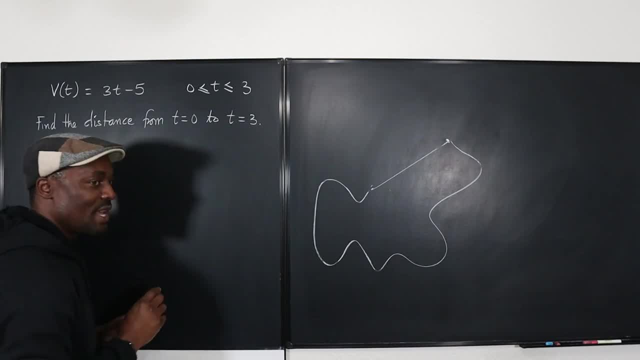 left where you were before. so what do you do? actually, the integration option is the correct option, but with a tiny little absolute value modification. so distance is the integral from 0 to 3 of the absolute value of the velocity- remember that okay- of 3t. 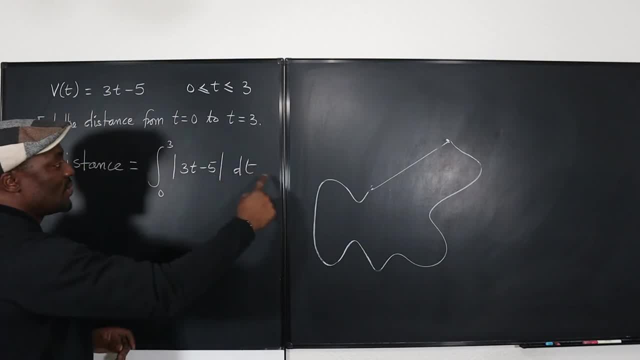 minus 5. and this is where many students get stuck, because once you put absolute value bars for definite integrals, you're going to get a number which is going to be positive, because you're going to get a number which is going to be positive, because you're going to get a number which is going to be positive. 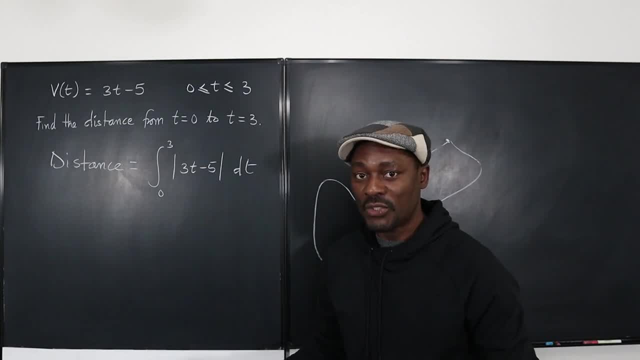 um, it becomes very iffy, okay. so just watch the rest of the video and know how to take this integral. and what's important is, you just need how. you know how. you need to know how to break this down, because once you're able to break this down, you can get your answer. so let's break this down. 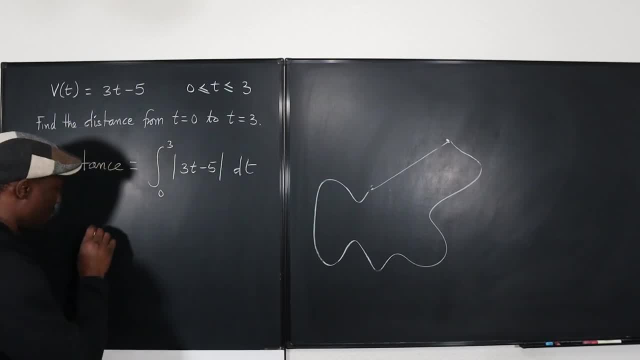 quickly. you see this integral- okay, could be the same thing as this- is equal to the integral from 0 to 3 of this function. let's see what this function looks like. this function, because it's an absolute value function, is something like this: and that's, that's terrible. okay, something like this when this function is: 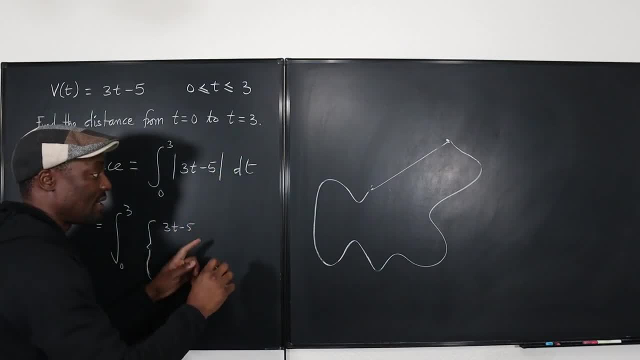 positive. you're just going to say it's 3t minus 5 when 3t, when 3t minus 5 is greater than or equal to 0. that's the definition of an absolute value function. it is what you see when that value is. 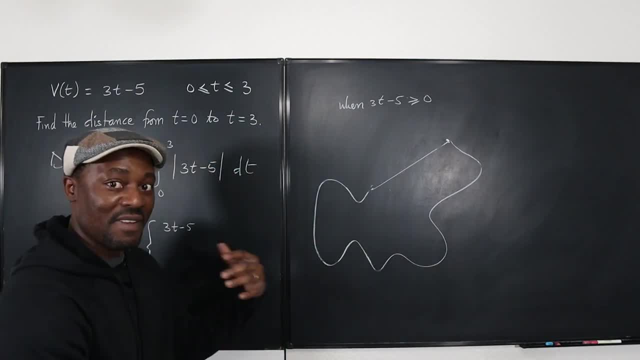 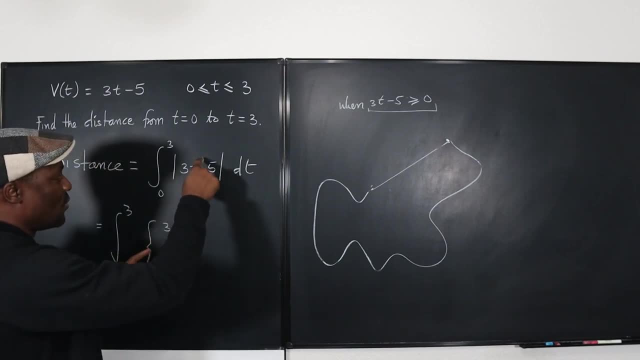 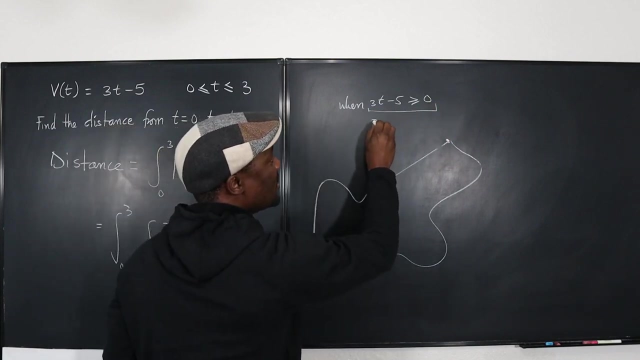 positive. it is the negative of it when that value is negative. so here you just need to quickly solve this inequality so that this function will have this value when this value is greater than 0. and when is this greater than 0? it means 3t is greater than or equal to 5. 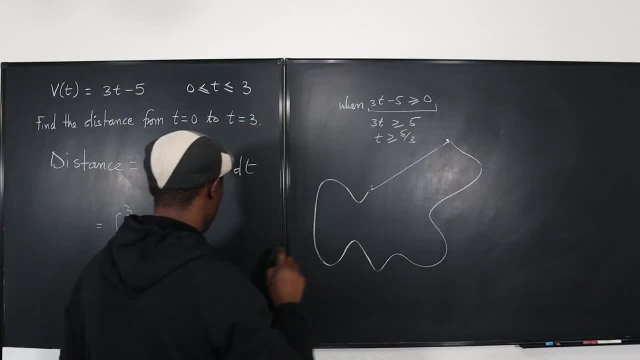 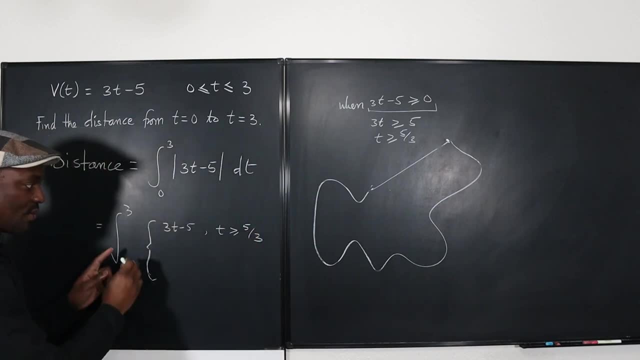 which means t is greater than or equal to 5 thirds. so what you write here is for t greater than or equal to 5 thirds. okay, you're integrating this dt. i'll have to write dt somewhere in the right here, okay, or the other option is going to be the negative version of this: 3t minus 5. 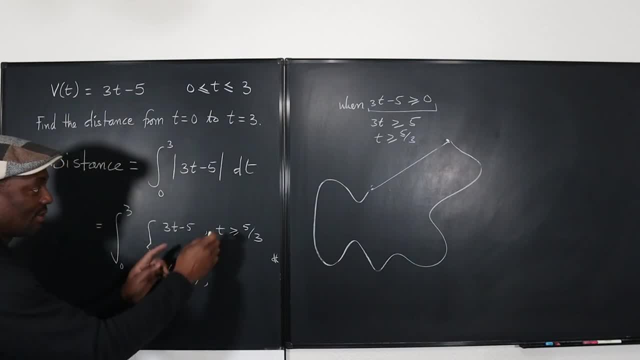 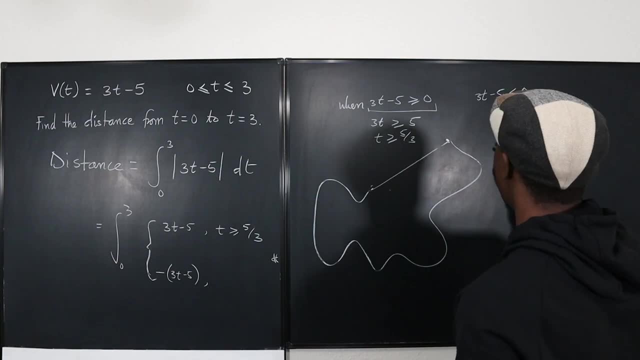 when this expression here is less than 0. so we do the other option. when 3t minus 5 is less than 0, that's the negative version, and when this is less than 5, we solve it. we're going to have, it's just. 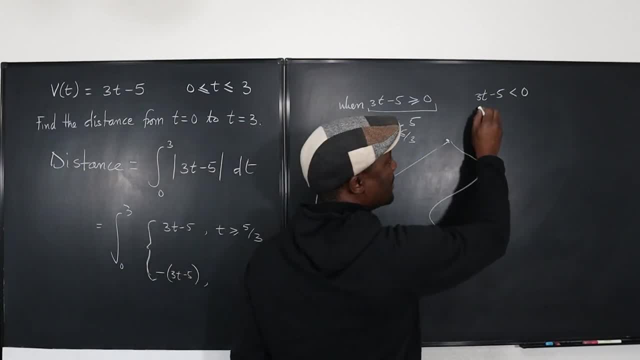 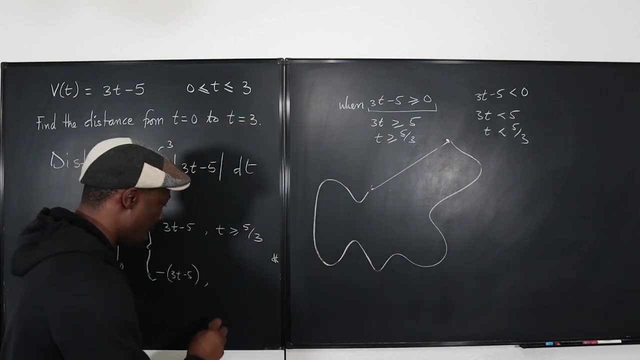 whatever is the contrary of this one. so we have 3t less than 5. t is less than 5 thirds. once you get this, you just change this to less than okay. so this works when t is less than 5 thirds. okay, and that's it, dt. let's move this back a bit. 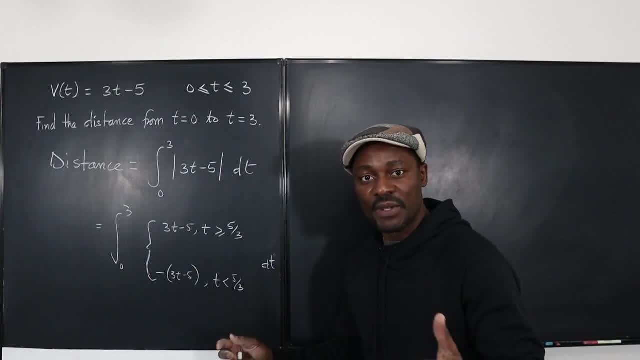 so this is the most difficult part- is you being able to break this down and expressing what t will be. you see how i was able to establish this. whatever, when you take an integral of absolute value function, you leave it the way it is, and what is here is greater than or equal to zero. you switch the sign, you put a sign behind it. 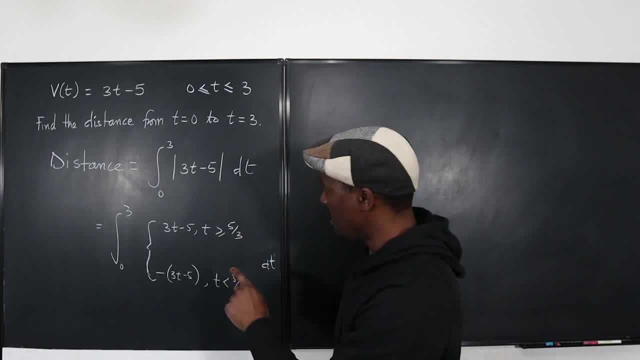 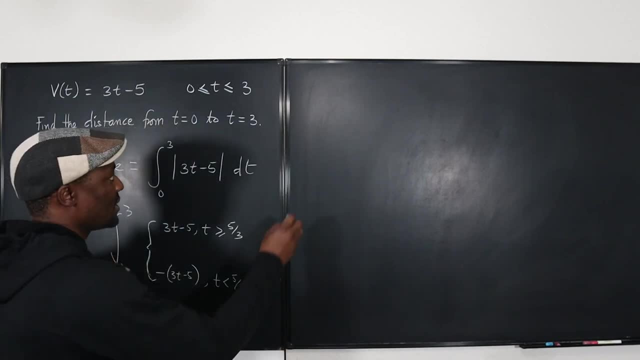 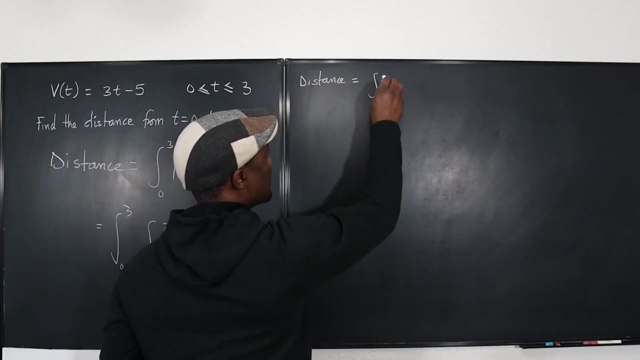 when it is less than or equal to zero, and you solve those inequalities to know what t will be. so now we can take our integrals. they're going to be in bits, so let's go. our distance will be equal to the integral. now look, we cannot integrate this function. let's put this function. 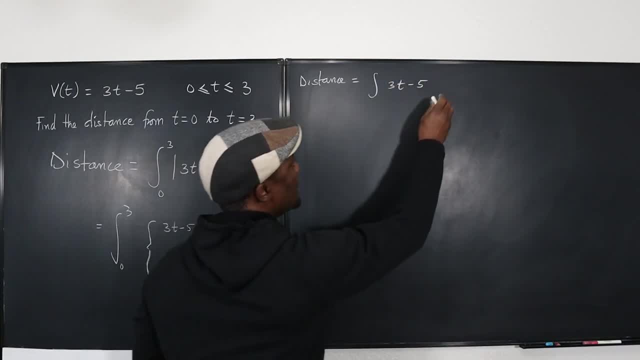 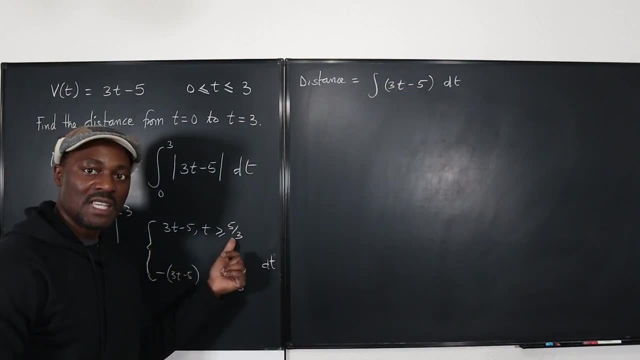 here, 3t is less than or equal to 0 and what is here is greater than or equal to 0. you switch the sign. you put a sign behind it: t minus 5 dt. you see, this function here is only relevant when you're dealing with values of t. 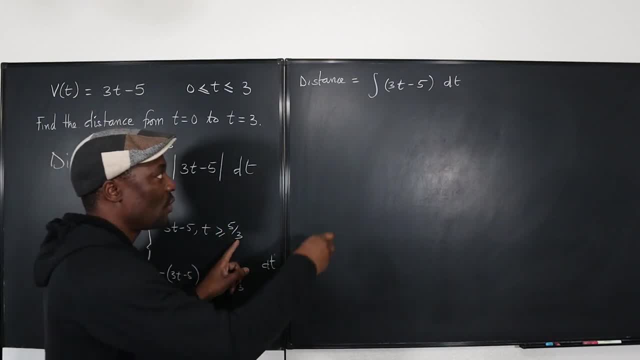 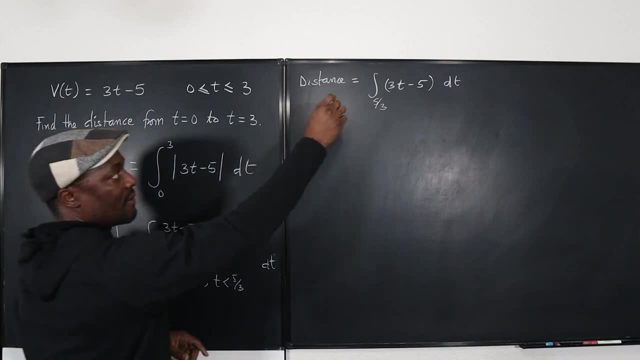 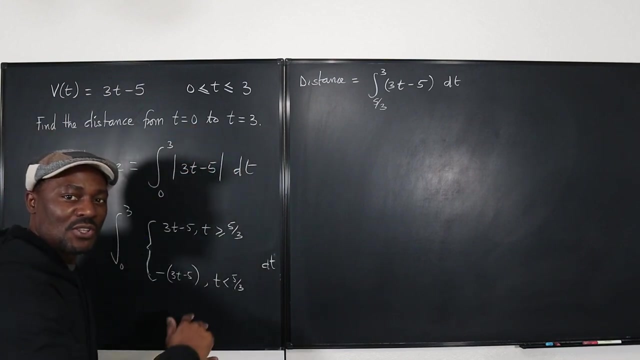 greater than or equal to 5 thirds. so you can only integrate from 5 thirds if you're using this to the maximum, which is 3, but when you go below 3 because you're starting from 0, so anything from 0 to 5 thirds you'll be. 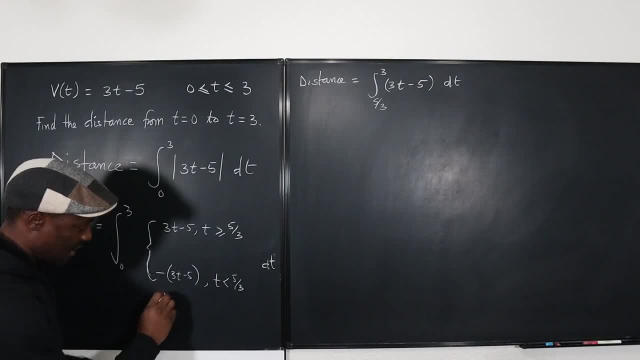 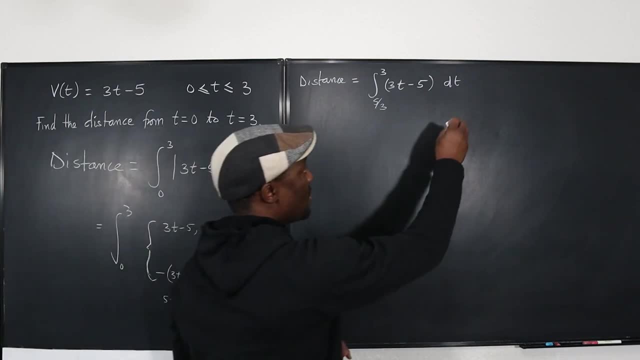 using this other integral, so you can only integrate from 0 to 5 thirds. if you're using this other integral, any function- and you see this function- can be written as 5 minus 3t. it makes it easier for you. just distribute the negative. this is what you get. so that's what i'm going to write here, plus this. 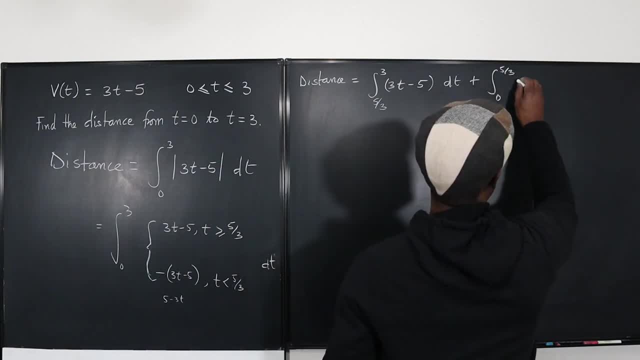 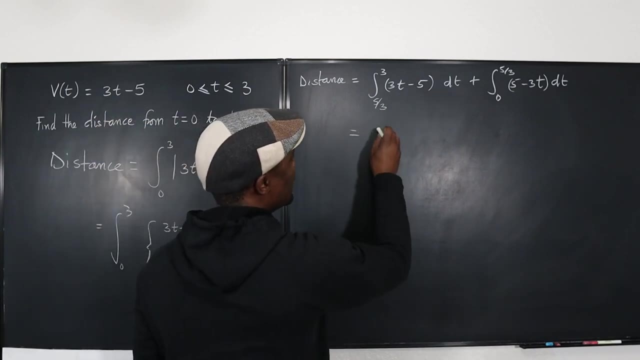 integral beginning from 0 to 5 thirds of 5 minus 3t dt. so that's all we've got, and now we'll see what our answer is going to be. let's do the integration. so this is going to be: let's integrate this. 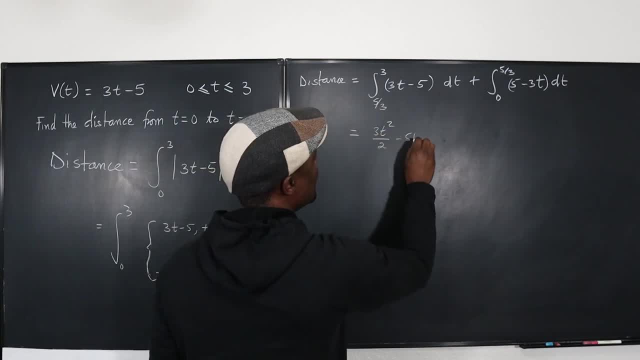 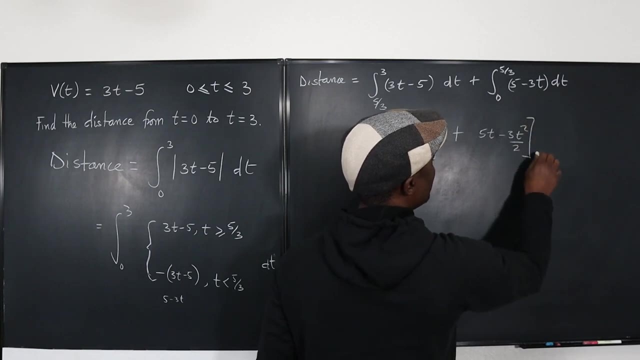 to be 3t, squared over 2 minus 5t, evaluated from 5 thirds to 3.. Plus, if we integrate this, this is going to be the same thing: 5t minus 3t, squared over 2, evaluated from 0 to 5 thirds. Okay, let's. 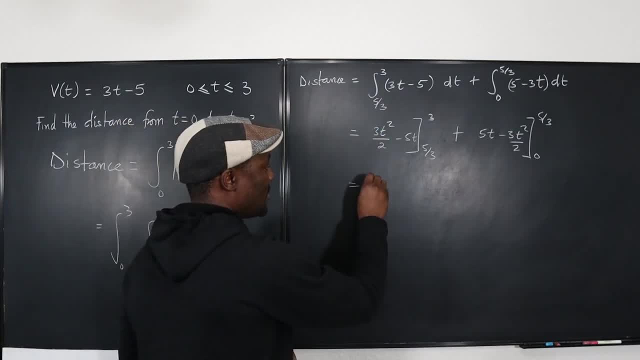 evaluate this. So this is what I do. I write the fraction first, 3 over 2, and I open a parenthesis and I plug in 3 here. What is 3 squared? It's 9 minus. I'm going to plug in 5 thirds here. So 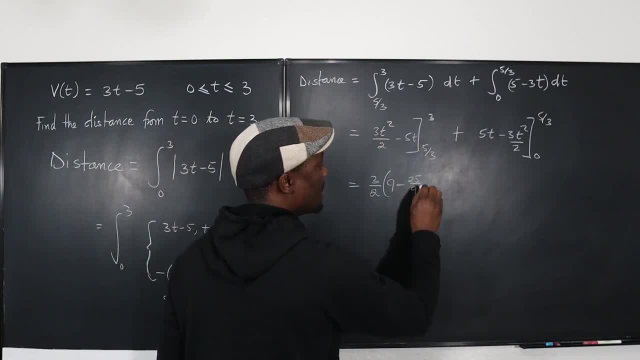 what is 5 thirds squared, It's going to be 25 over 9.. I'm done with this side. Okay, plus or minus 5 times. I'm going to plug in 3, it's going to be 3.. I'm going to subtract. I plug in 5 thirds. 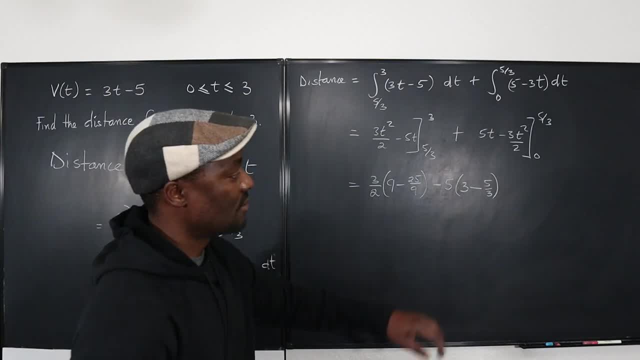 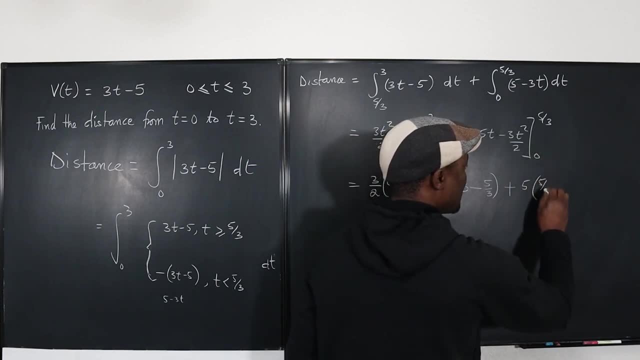 it's going to be this. Okay, I'm done with that. Let's go to the next one, Plus. here I do the same thing: 5, it's going to be 5 thirds minus, I plug in 0, it's just 0.. And the last one is going to be minus 3 over 2, I plug in 5 thirds. 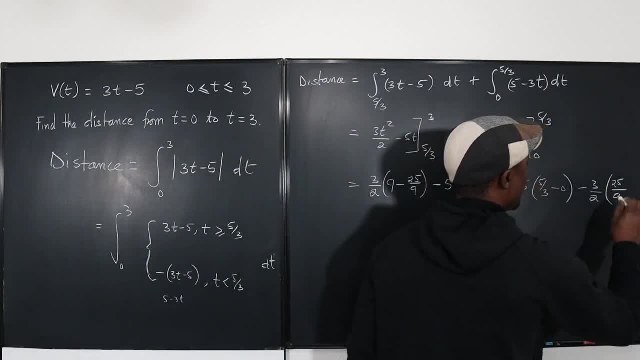 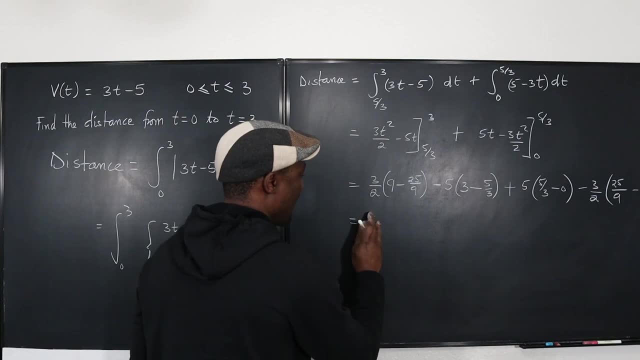 squared, that's 25 over 9,, 25 over 9, and then I plug in 0,, it's just minus 0.. Okay, next step. this is going to be 2 thirds, sorry, 3 halves, 3 halves of. 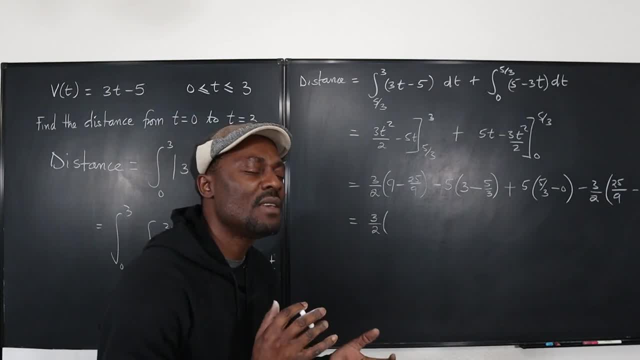 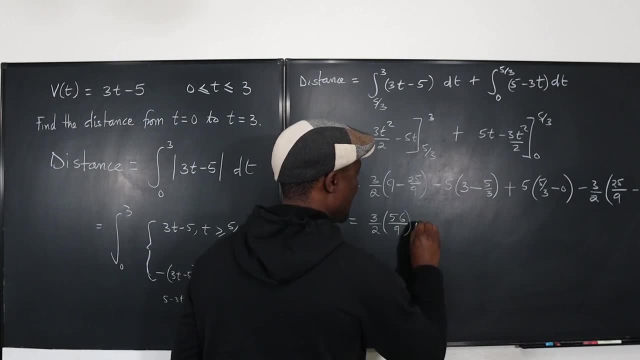 this is 81 minus 25, that's going to be 56. Okay, that's 56 over 9 minus 5 times. this is going to be 9 minus 5, what's that? That's 4,. that's 4 thirds. Okay, plus, this is 5 times. 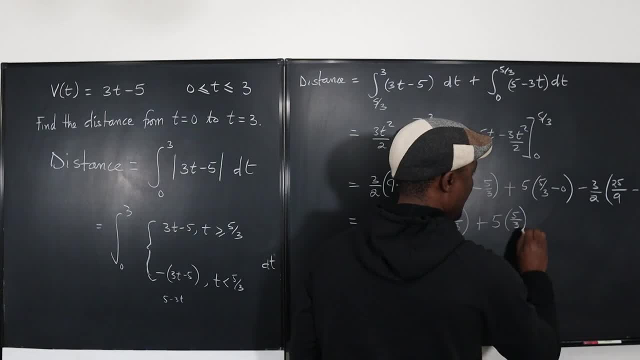 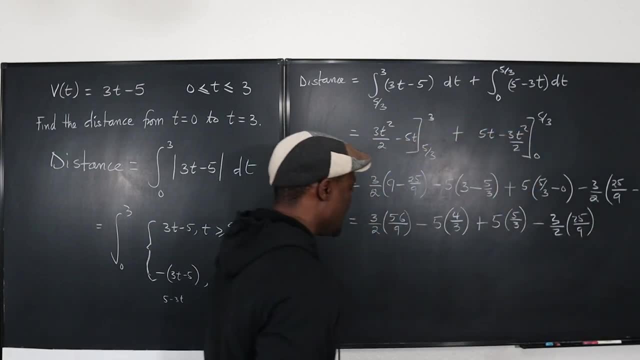 5 thirds minus 2, minus 3 halves of 25 9s. Okay, let's now see how this works out. This 3 is going to cancel some 3 here, so you have 3 left. This 2 will reduce this to 28,. so it's 28 over 3, so this is 28 over 3, minus. this is going to be. 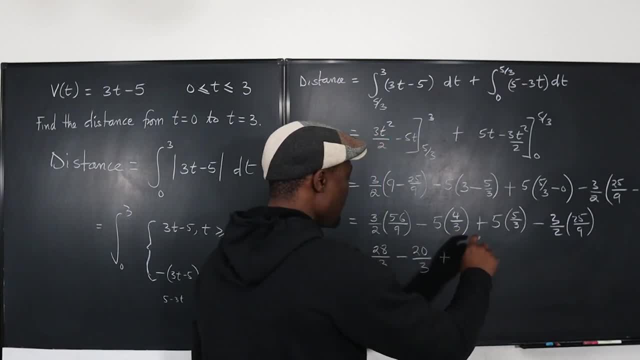 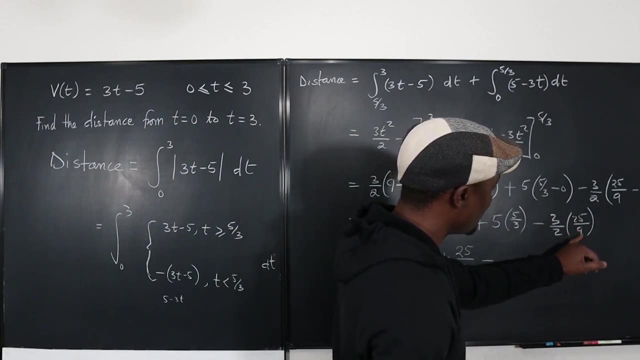 20 over 3, plus. this is going to be. what would this be? 25 over 3, and this is going to be minus. let's go. this 3 will cancel this. what would it be? That's just 3,, so that's 25 over 6, 25 over 6.. 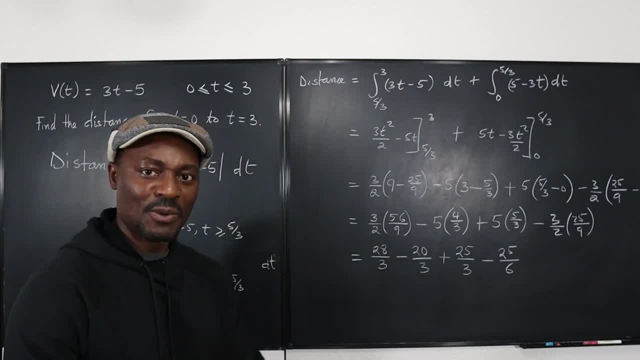 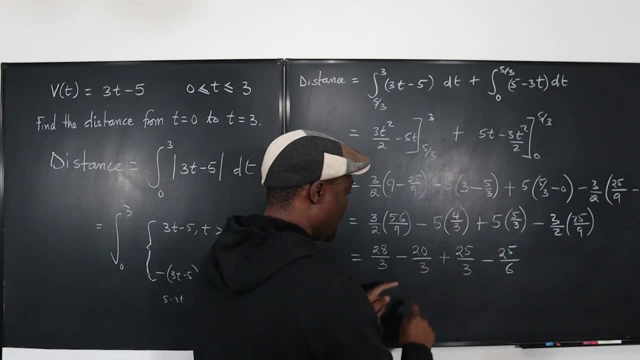 Okay, whatever you get here will be your answer. Let's deal with all the 3s first, all the ones that have 3s. so I'm going to deal with these. This is 28 minus 20, that's going to be 8,. 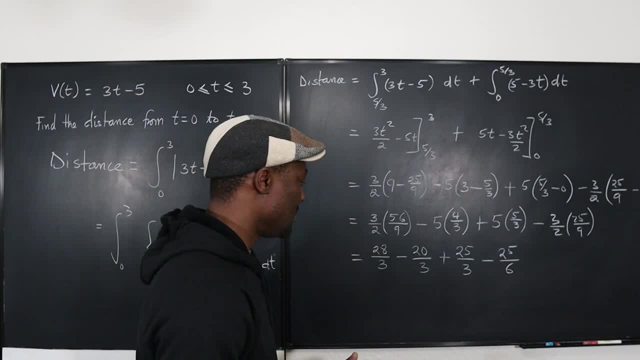 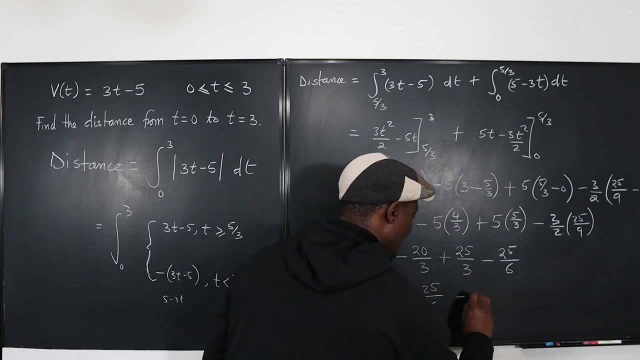 8 plus 25 is going to be 33, so this is going to be 33 over 3, minus 25 over 6.. Well, let's see I can make this 66 over 6,, that's 66 over 6, minus 25 over 6.. 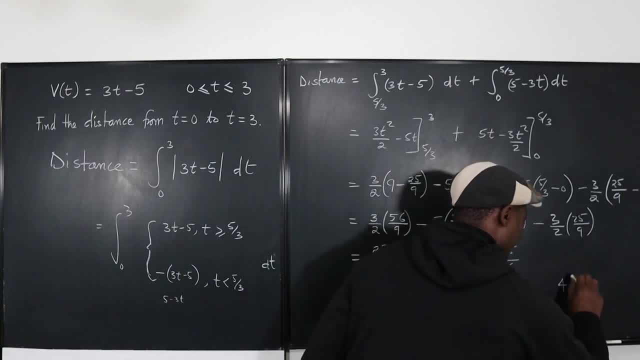 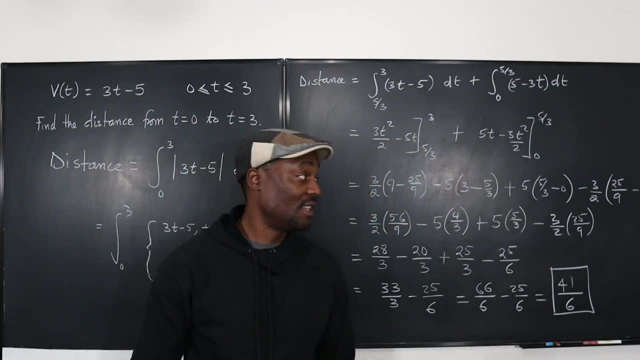 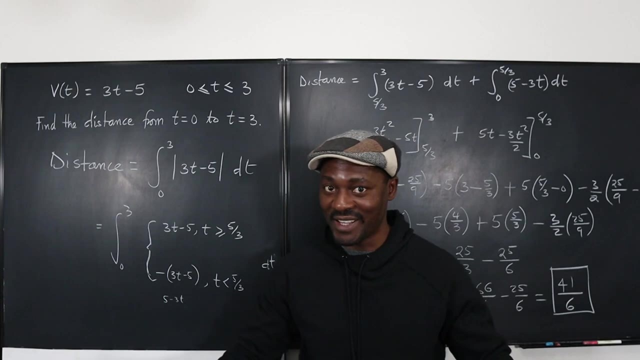 Ladies and gentlemen, 41 over 6 is the answer. It's different from what you would do if you didn't go through this step. So this question looks innocent, but the process is not that innocent. it's wicked. Don't stop learning. because those who stop learning have stopped living Bye-bye.